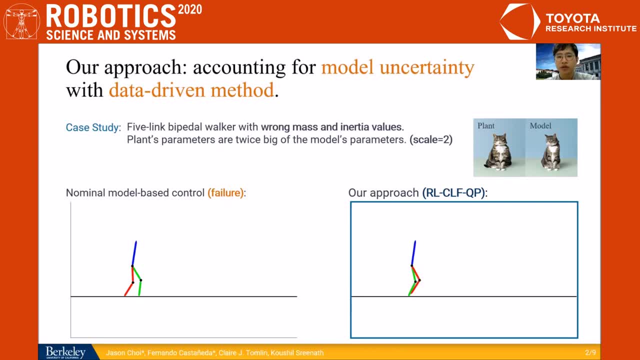 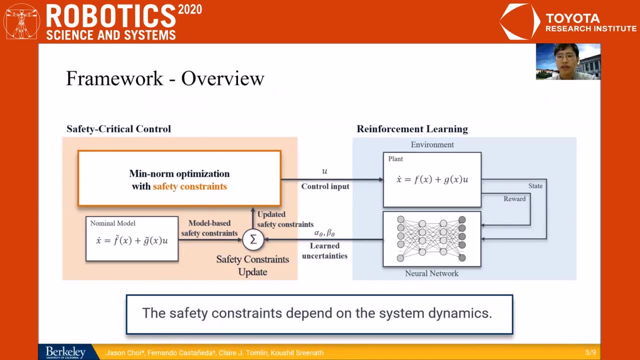 to learn this model uncertainty and obtain a stabilizing controller. This is the framework of our work. It consists of a mineral optimization problem that is solved online, which includes stability and safety constraints, But these constraints depend on the dynamics of the system. That is why we need to learn the model uncertainty terms. 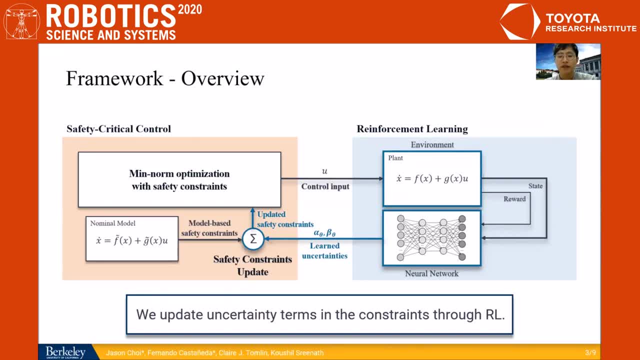 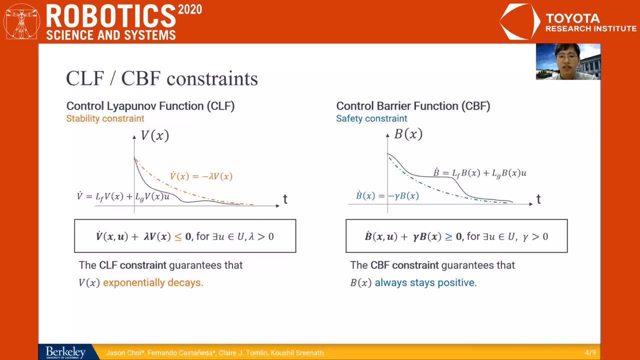 and use them to create estimates of true stability and safety constraints. These constraints are based on Control-Yakono Functions and Control-Bearer Functions. The CLF constraint guarantees that the input uptake is obtained from the optimization problem will exponentially stabilize the system. In contrast with the CBF constraints, we guarantee set invariance and therefore safety. 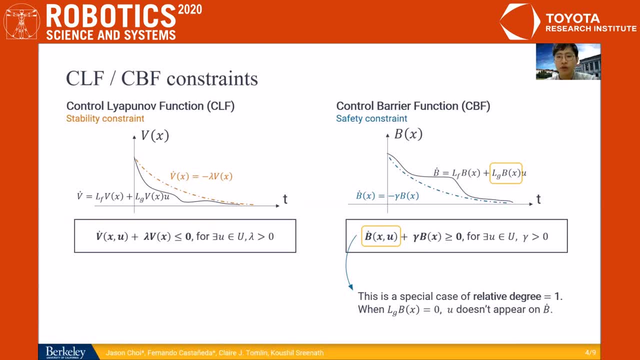 However, this formulation of CBF can only be used to enforce safety constraints in which the input appears at the first time derivative. We call this having relative degree 1.. For many applications, this formulation is not enough and we need to extend it to higher relative degrees. 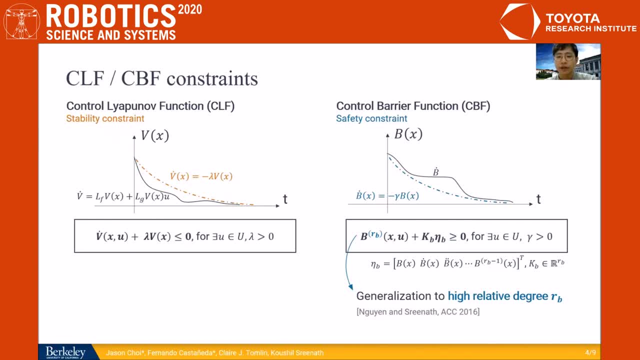 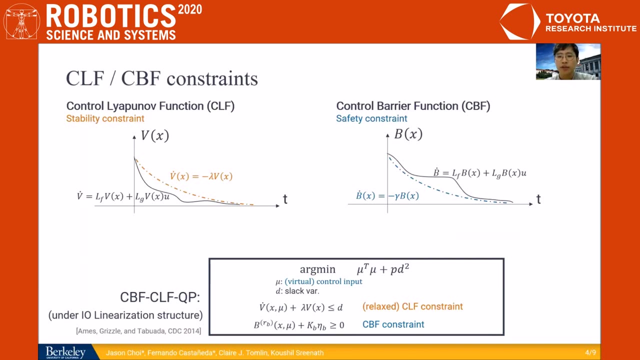 Let's see how the safety constraint looks for a general relative degree Rb. We now integrate these constraints in the mineral optimization problem. We relax the CLF constraint to give preference to safety over stability in case of conflict, And this is the final form of the mineral optimization problem. 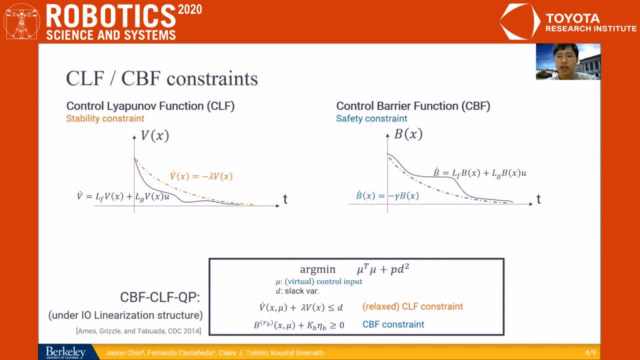 which solves for a virtual control input of a feedback input-output linearization controller. But, as we have said before, these constraints depend on the system dynamics, so if our model is wrong, this constraint will not manage to stabilize and keep the system safe. 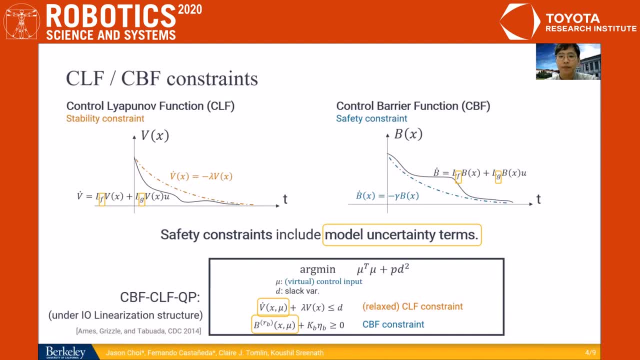 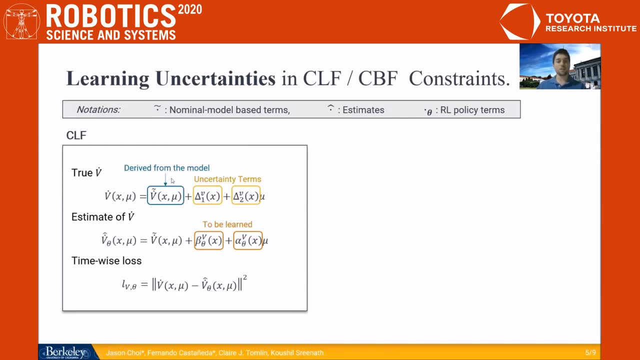 And now I'd like to hand over to Fernando. Thanks, Jason. We can actually express the true V-dot as a sum of a model-derived term expressed with a tilde and this control-defying term with uncertainties: delta1 and delta2.. Our objective is to build an estimator V-dot-hat by learning the functions alpha, theta and beta. 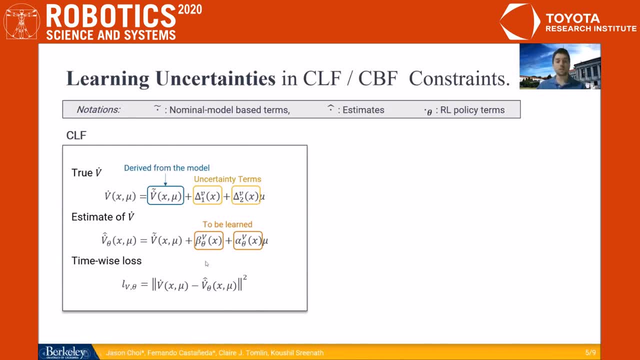 theta. For that purpose we will use this list-definition For the R-derivative of the CBF. we follow exactly the same approach, since the true value of the derivative is again a sum of a model-derived term and uncertainty terms. So we build an estimator of the true derivative of these four.